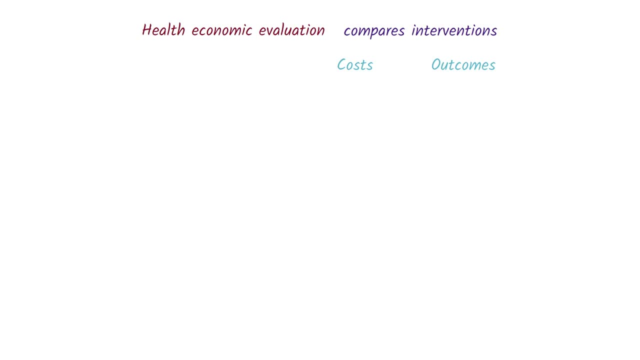 on the basis of their costs and outcomes. There are four main types of economic evaluations: cost minimization, cost effectiveness, cost utility and cost-benefit analysis. They all compare costs with outcome, but do so in different ways. Let's have a look at the different types of costs. first, Direct costs are costs that are directly 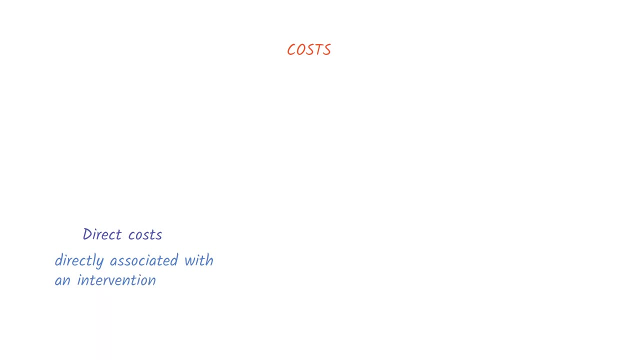 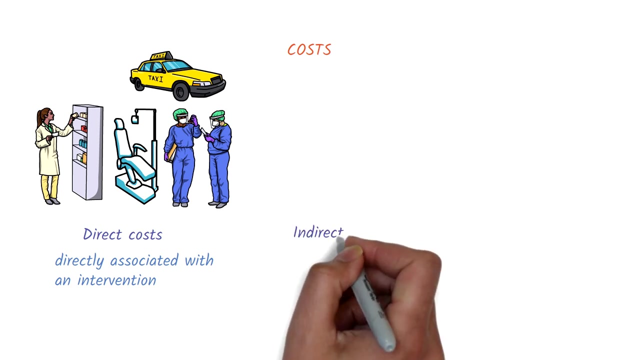 associated with intervention, For example, the cost of medicines, the cost of equipment like x-ray machines, salaries of healthcare staff or the cost of transport to the health center. Direct costs are the main focus of most economic evaluations. Indirect costs are costs associated. 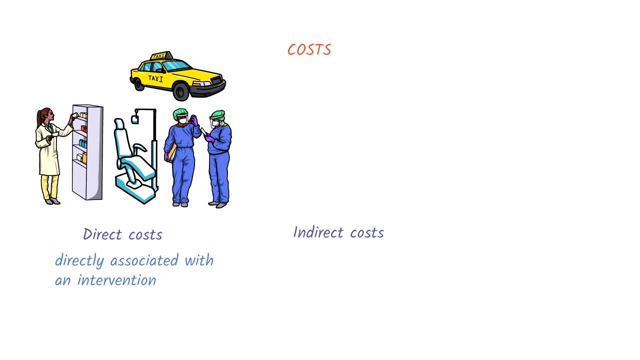 with reduced productivity due to the illness or its treatment. An example is missed wages because of not working due to the illness. Intangible costs are subjective, such as pain, suffering or grief due to the illness or treatment. These costs are quite hard to put a monetary value on. 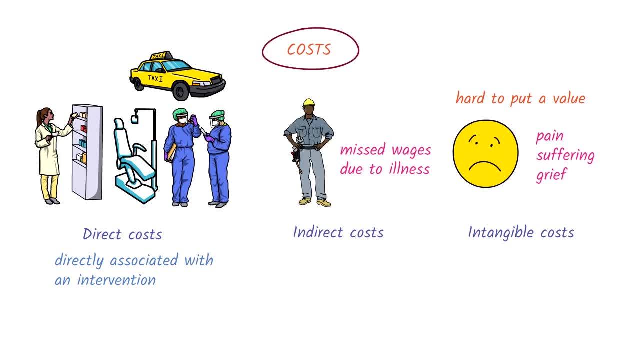 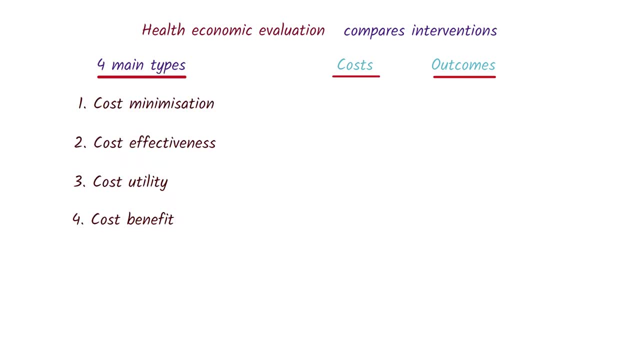 That's a look at the different types of costs. Now let's take a look at the different types of economic evaluations. The first type of economic evaluation is a cost minimization analysis. This type of analysis is used when the product or outcome is the same. 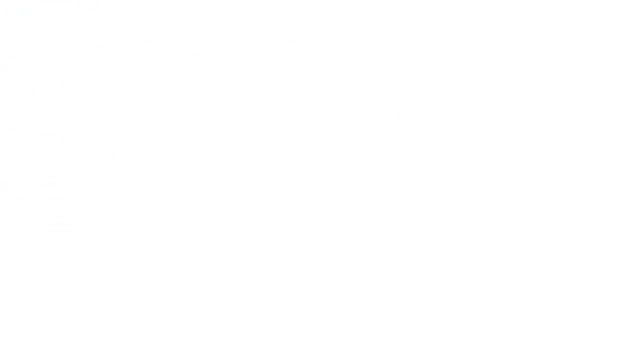 and what we're comparing is the cost. For example, let's say we're comparing blood pressure reducing medications that are made by different manufacturers and have different prices. In a cost minimization analysis, because the medicine is the same, we simply compare the. 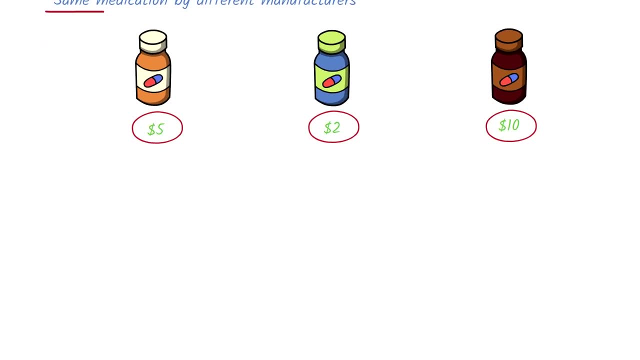 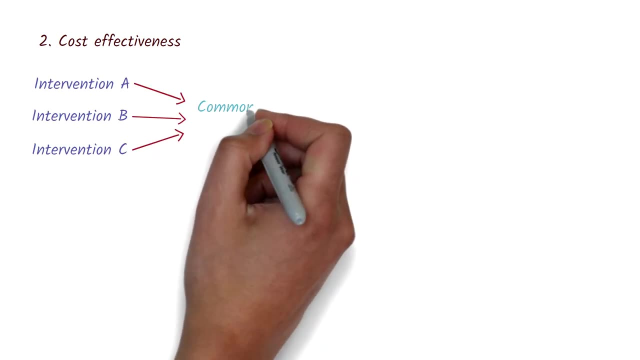 costs. The second type of analysis is a cost effectiveness analysis. This is used when a product is made by different manufacturers and has a different cost. For example, we're comparing different interventions that have a common health outcome. Examples of health outcomes are reduction. 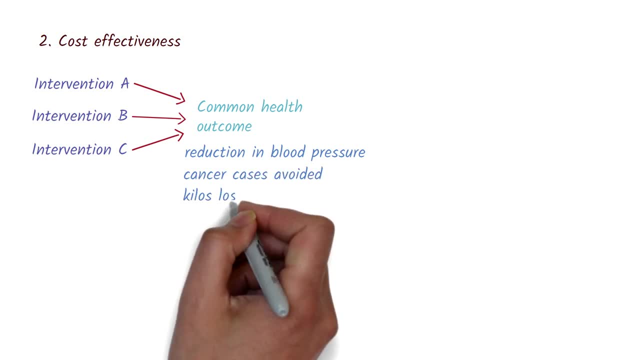 in: blood pressure, cancer cases avoided, kilos lost or life years gained. These are called natural units. Let's take a look at an example. Let's say we're comparing two different interventions to reduce weight: A diet program and weight loss medication. The health outcome. 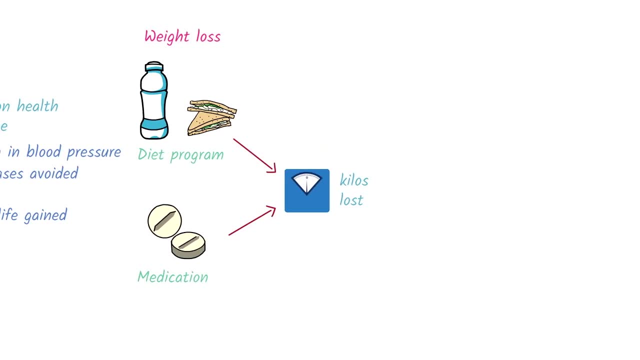 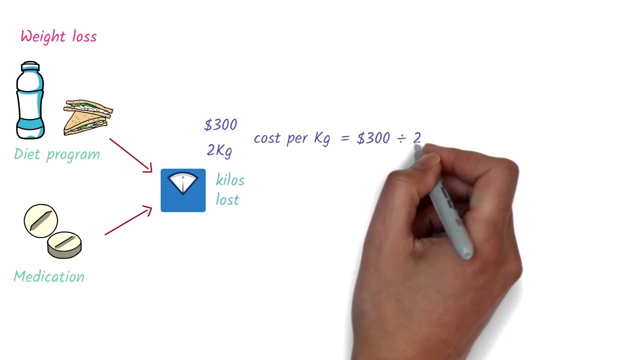 we're interested in is how many kilos have been lost. The diet program had a two kilogram weight Loss and cost $300.. The cost per kilo lost is $150.. This is called a cost effectiveness ratio. Let's compare this with a medication-based program that leads to a weight loss of three kilograms. 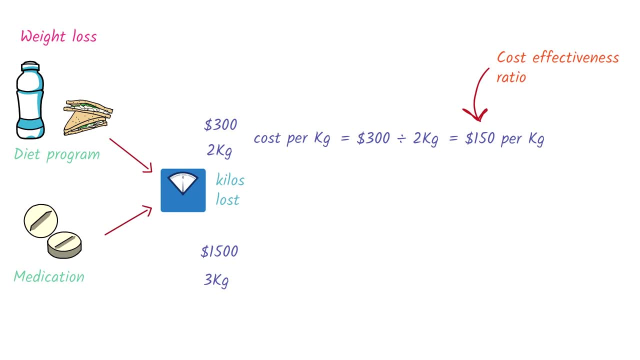 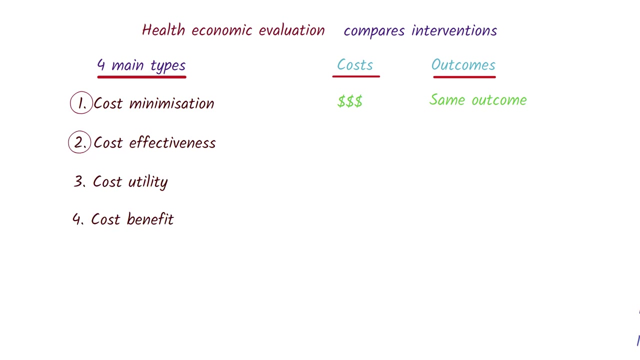 but costs $1,500.. In this intervention the cost per kilo lost is $500.. So in this scenario the diet-based program is more cost effective compared to the medication-based program. So a cost-effective analysis compares the cost per natural units for different interventions. 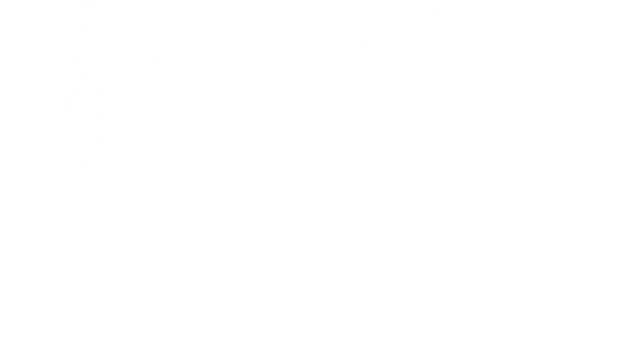 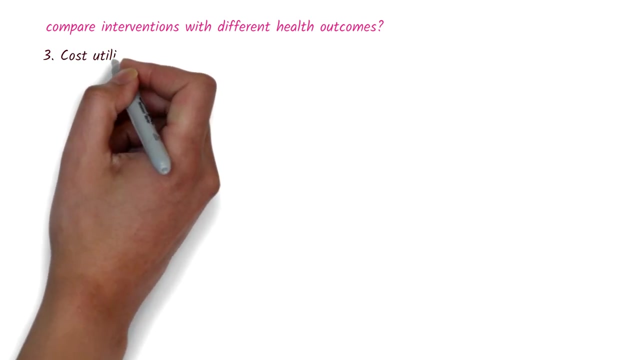 But what do we do if we want to compare interventions that have different health outcomes? For this we use a type of economic analysis called a cost-utility analysis. Let's have a look. Say we want to compare between drug therapy to reduce high blood pressure. 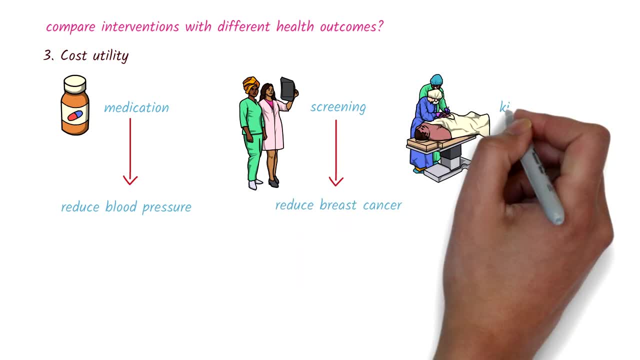 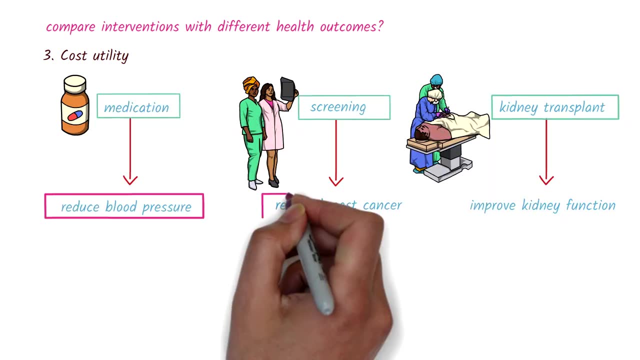 breast screening to reduce the number of breast cancer cases, and a kidney transplant for end-stage kidney disease to improve kidney function. These are different health interventions that have different health outcomes, So in order to compare these different interventions, we need to have a common outcome measure that can be applied to all these interventions. 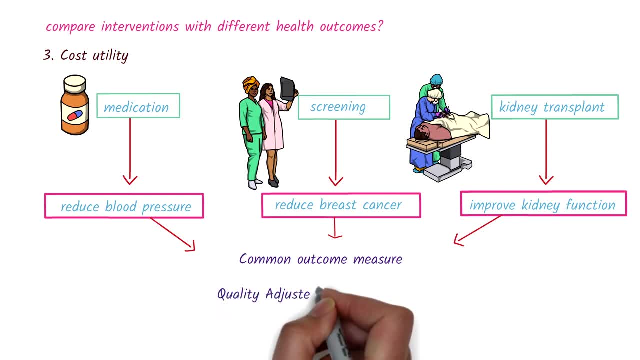 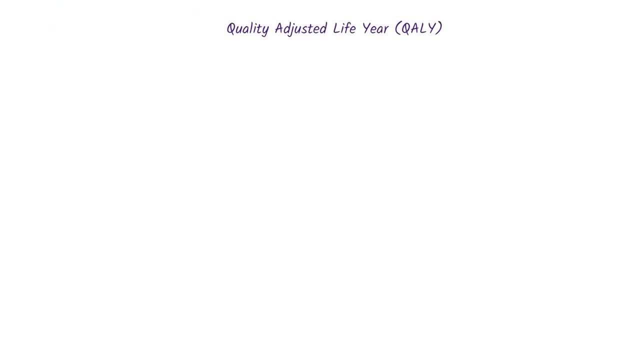 The measure that is most commonly used is called the quality-adjusted life year, or QALY in short. Let's have a look at what a QALY is. Health interventions Try to prolong a person's life by increasing the number of years a person lives, and they also try to improve the 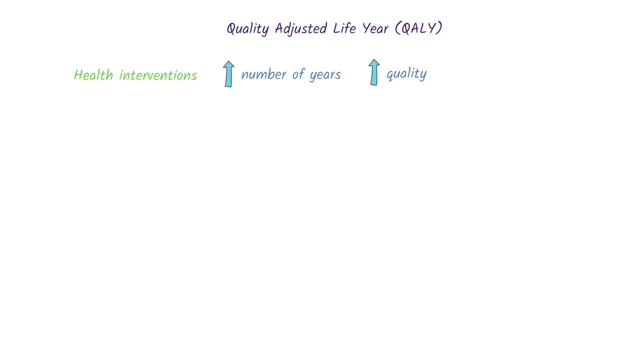 quality of those years lived. A quality-adjusted life year is a combined measure that takes into account both of these aspects. A QALY is calculated by taking the number of extra years gained as a result of the intervention and multiplying it by the quality of life of those extra years. 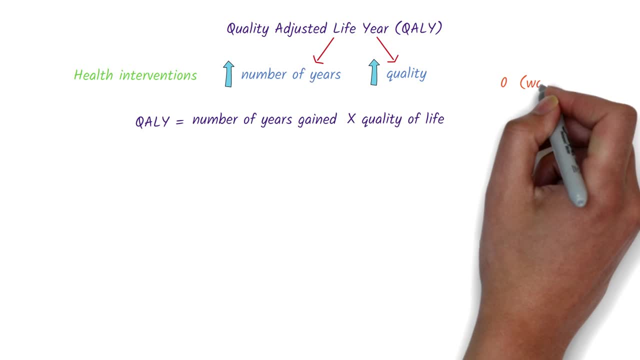 Quality of life is graded from zero to one, from zero being the worst possible health state and one being the best possible health state. There are many different ways to determine these gradings. They usually involve asking people how they rate their quality of life. 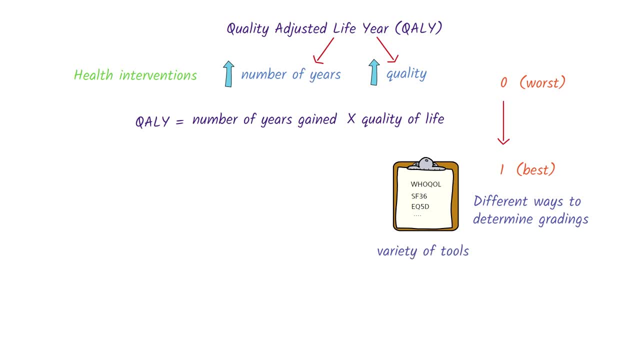 A variety of tools can be used for this. Measures such as QALYs are called health utility measures, because they measure an individual's preference for different health outcomes. Let's have a look at an example. If an intervention leads to a person living five years in perfect health, 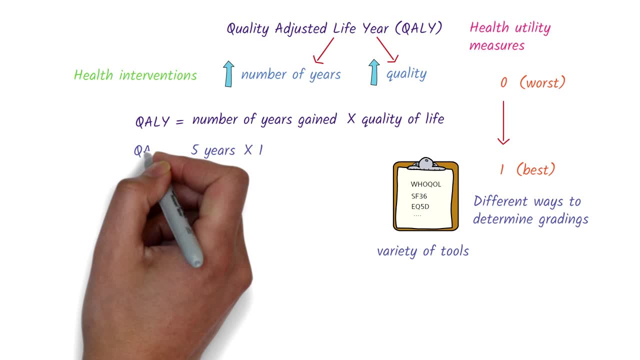 a health utility of one, then the number of QALYs gained as a result of this intervention is five. Similarly, if an intervention leads to a person living an extra five years, but with a quality of life of 0.2,, 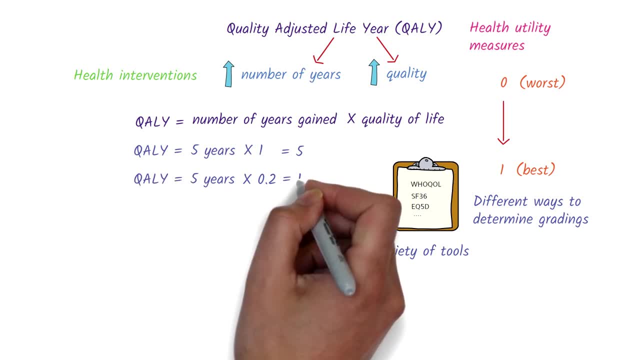 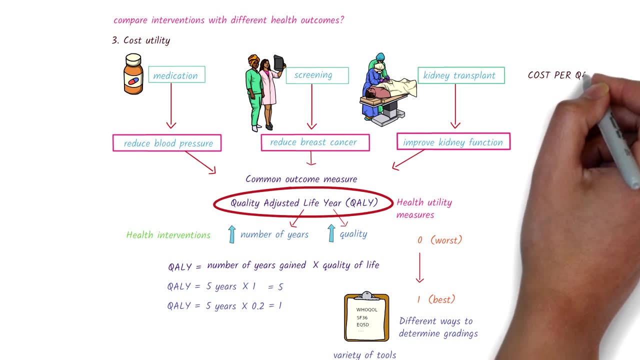 then the QALYs gained as a result of that intervention is one. Now that we have a common outcome measure, a QALY, we can compare the cost per QALY across different interventions. So a cost utility analysis compares the cost of a utility. 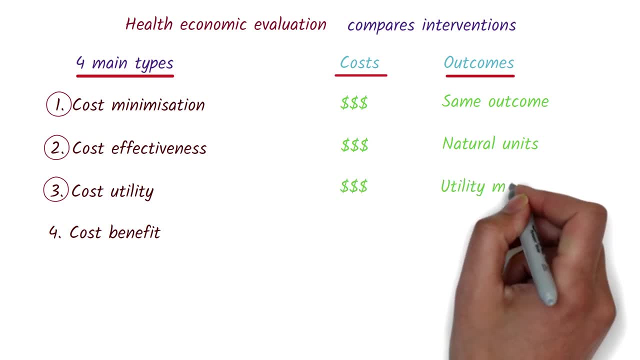 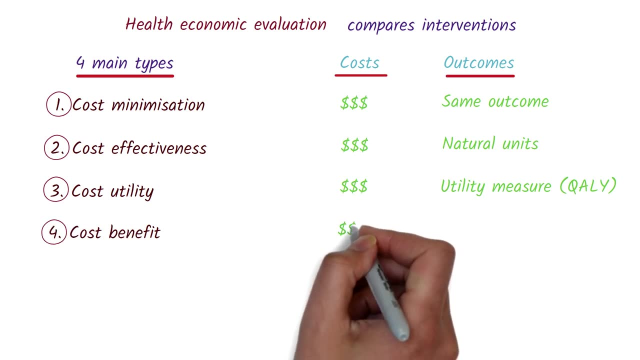 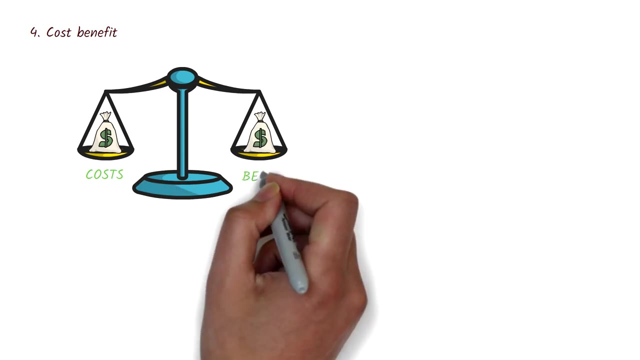 measure such as a QALY for different interventions. Now let's have a look at cost-benefit analysis. This type of analysis measures both the cost and outcome in monetary terms. A cost-benefit analysis tries to account for all costs and all. 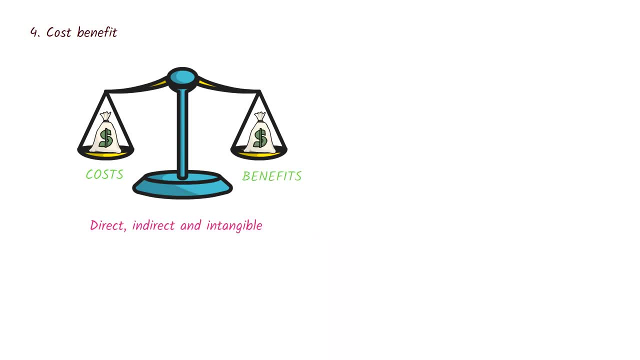 benefits – direct, indirect and intangible. To calculate benefits, a variety of tools can be used. The willingness to pay method determines the value that people attach to health outcomes, For example by asking people how much they're willing to pay to have the benefits of the. 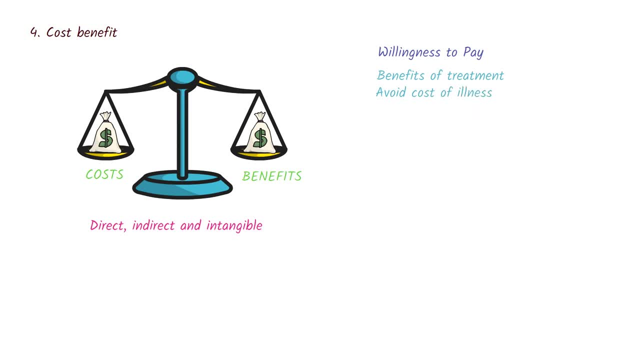 treatment or to avoid the costs of illness. The human capital method places a monetary value on the person's life. The value is based on the loss or gain of income due to the illness. Although this type of evaluation is comprehensive, the data requirements can be quite high. 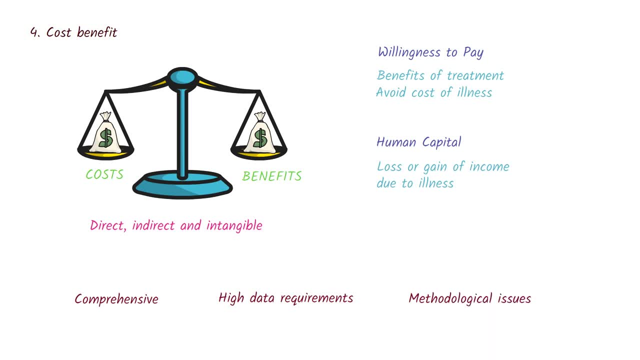 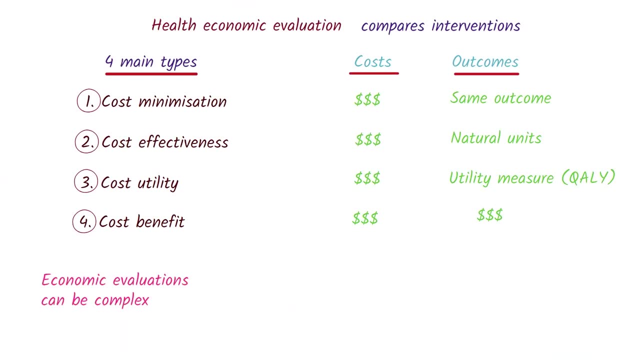 and there are methodological issues when it comes to determining a value on life and productivity. In reality, economic evaluations can be quite complex to do and require various statistical calculations and adjustments, such as stratification to adjust for different patient groups that might benefit differently from the interventions. discounting to account.